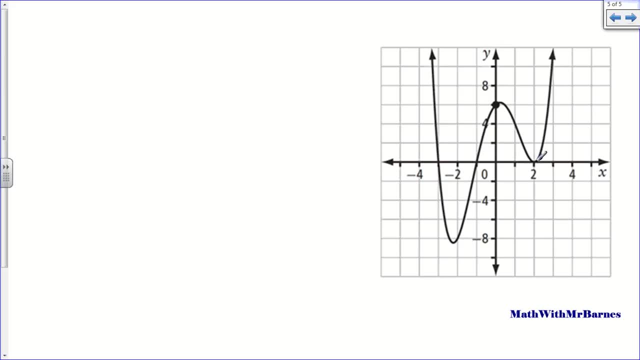 So I know it's a double root because it comes down and it bounces off the x-axis. That's how I know it's a double root. So what I generally do is I list out my x-intercepts for this. So my x-intercepts are so we just listed them out. so negative 3,, negative 1, and 2.. So from that I want to be able to write my factors. So I'll generally write them like this: 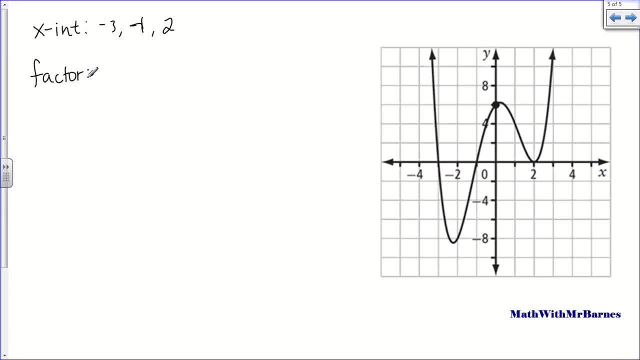 So my factors are this: So from 3, or negative 3,, I get x plus 3.. So remember, your factors are always the opposite signs of your x-intercepts. From negative 1, I get x plus 1.. And from 2,, being that it's a double root, I have x minus 2,, the opposite sign. 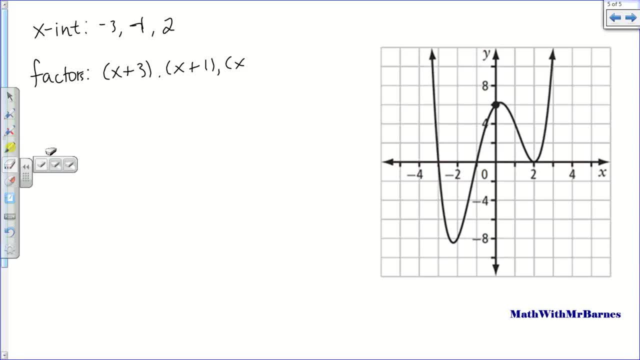 Let me fix that up a bit. So I have x minus 2.. And then that, because it's a double root, I get x plus 1.. So if I want to find the equation of this guy, I'll write it, as the only thing I don't know is what my leading coefficient is. so a 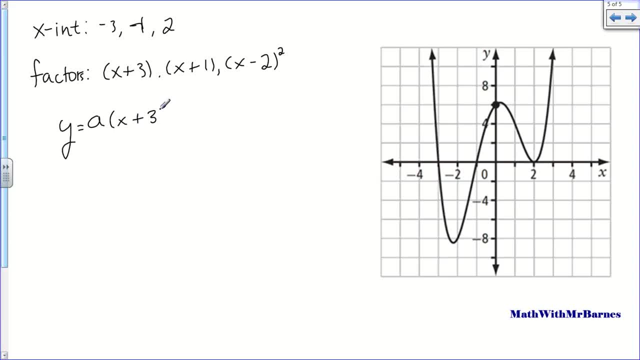 So I'll write out my factors just like this, And again, there's no real particular order to do it, I just, you know, list them out. Usually I'll put my squares and my cubes, if there's any last. 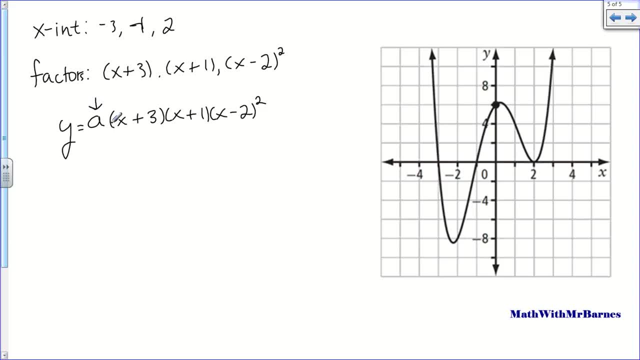 The next thing I need to do is I need to figure out this a value. So what I usually do is I look for a point on the graph. Usually, the y-intercept is usually a good candidate, So that y-intercept is 0, 6.. 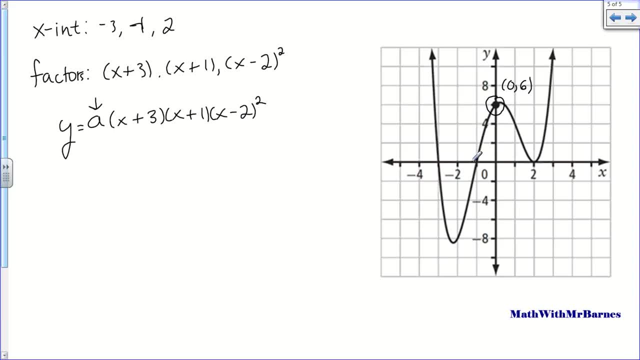 Now you can find another point on the graph. This one looks like a pretty good point. You don't want to use an x-intercept. You want to use another point besides the x-intercepts. So what we do is we plug this in. 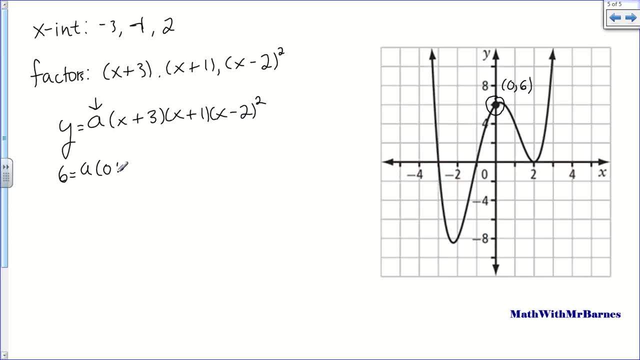 And we solve for a. So I have 0 plus 3,, 0 plus 1, and then 0 minus 2 squared. So what I have is 6 is equal to a, And I have 3,, 1, and then negative 2 squared. 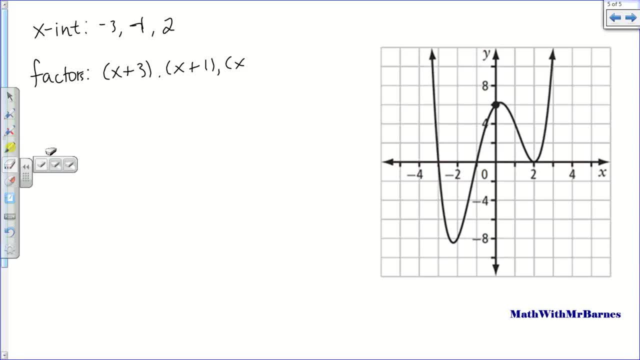 Let me fix that up a bit. So I have x minus 2.. And then that, because it's a double root, I get x plus 1.. So if I want to find the equation of this guy, I'll write it, as the only thing I don't know is what my leading coefficient is. so a 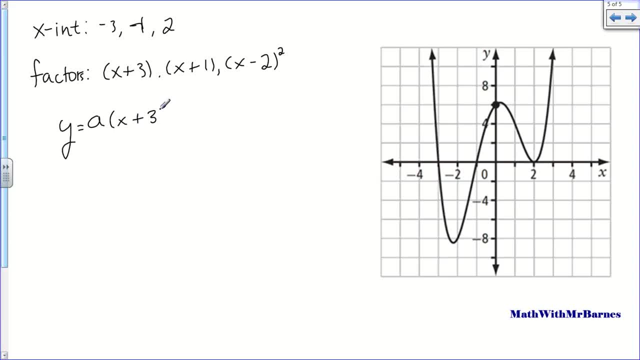 So I'll write out my factors just like this, And again, there's no real particular order to do it, I just, you know, list them out. Usually I'll put my squares and my cubes, if there's any last. 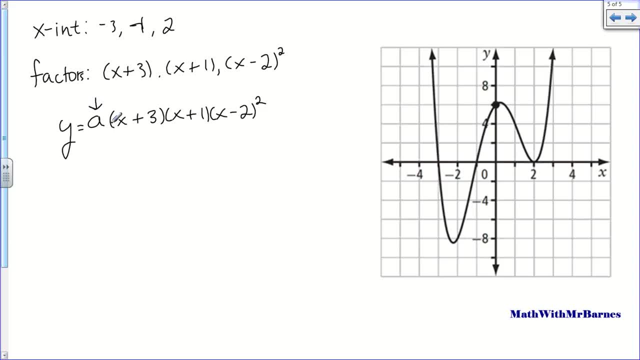 The next thing I need to do is I need to figure out this a value. So what I usually do is I look for a point on the graph. Usually, the y-intercept is usually a good candidate, So that y-intercept is 0, 6.. 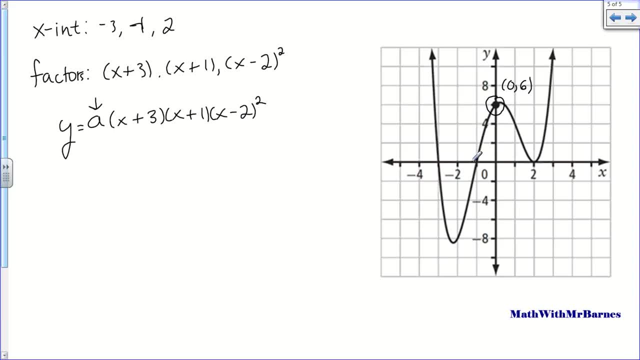 Now you can find another point on the graph. This one looks like a pretty good point. You don't want to use an x-intercept. You want to use another point besides the x-intercepts. So what we do is we plug this in. 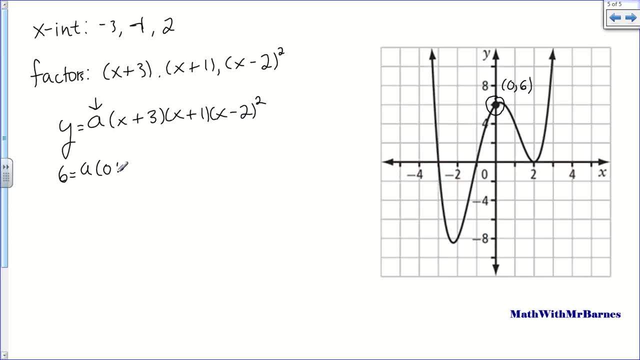 And we solve for a. So I have 0 plus 3,, 0 plus 1, and then 0 minus 2 squared. So what I have is 6 is equal to a, And I have 3,, 1, and then negative 2 squared. 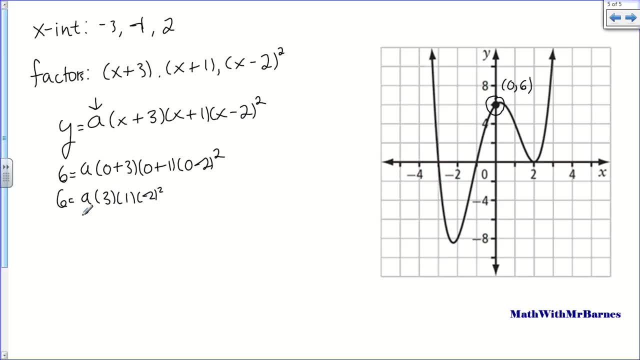 So that's going to be 4 times 3.. So that's actually 12.. So I have: 6 is equal to 12a. Divide both sides by 12.. And I have a is equal to 1 over 2.. 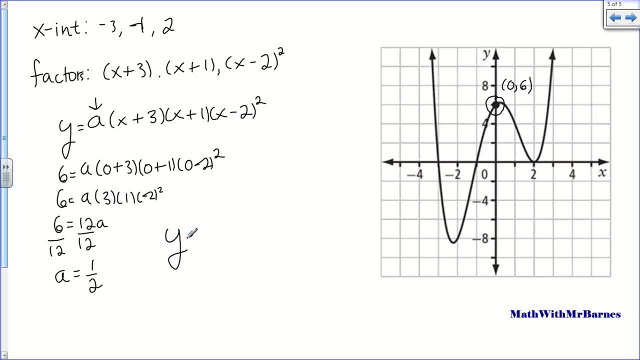 So now I can write my equation. So I don't need to like distribute this out or anything, guys, I just need to write this: This is the equation. I mean, it's not the, you know, it's not what we're used to seeing. 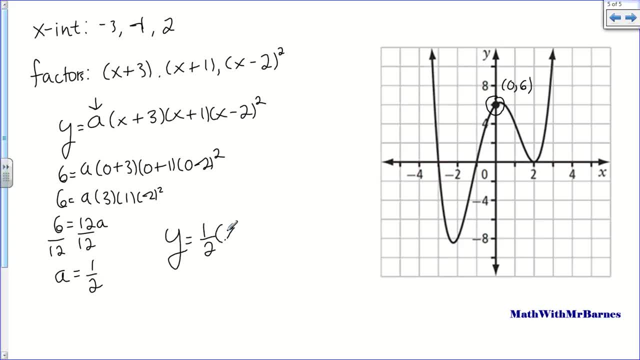 A lot of times we're used to seeing you know in expanded form. But if it's just asking for the equation, it's not asking for us to expand it. Why take the risk in expanding it, Especially in a test, if you don't have to? it's a complete waste of time.